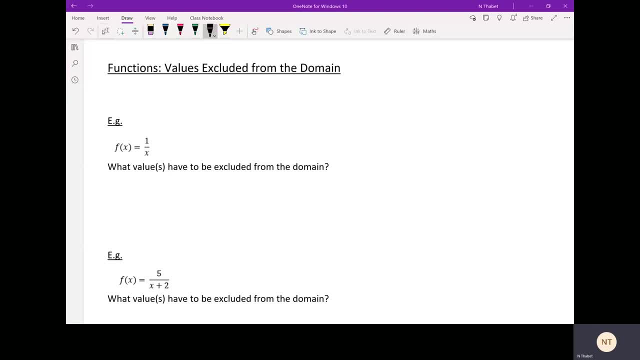 by 0.. Therefore, the value that x cannot be the value that has to be excluded from the input from the domain, is the value x equals 0. All other numbers will work except 0.. For the second example, again you've got a fraction and it's the function 5 over x plus 2.. 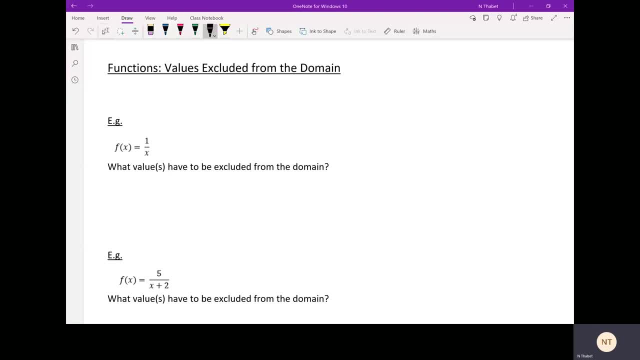 Well, we know that the whole denominator. so we know that x plus 2 cannot equal to 0, because if it equals to 0, then the division will not work. So what that means is that you're going to solve the equation to 0 equals 0.. x plus 2 equals 0.. If I solve this, I have to take away 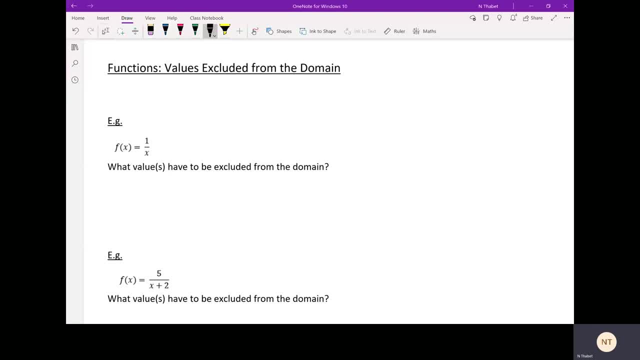 2 from both sides, and that gives me x equals negative 2.. x equals negative 2, is the value that has to be excluded from the input. Why? Because if you substitute it in minus 2 plus 2, that will give you 5 over 0, which cannot work. So x equals negative 2. 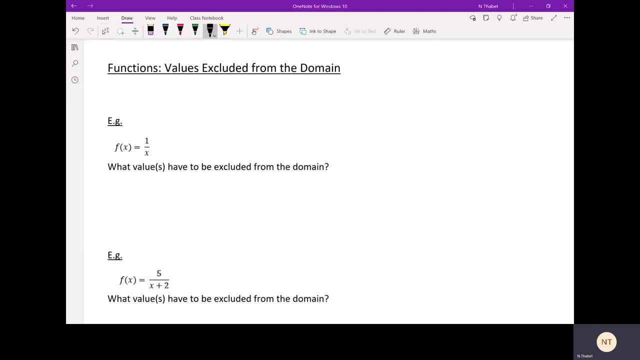 is the value that has to be excluded from the domain. Now this, The third example, is a little bit different, because instead of a fraction, you have a square root. Now, if you remember, square rooting is the opposite of squaring. 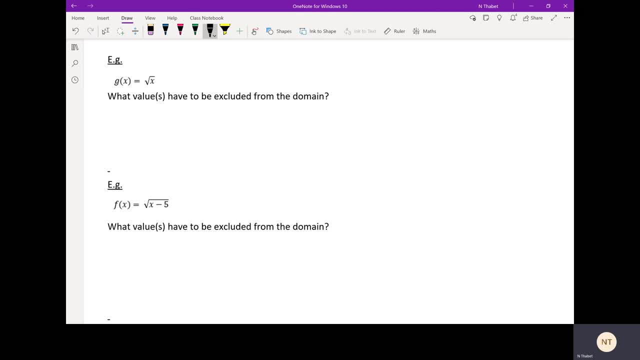 And whenever you square a number, you always get a positive. So, for example, 3 squared is 9, but negative 3 squared is also a positive 9.. So if square rooting is the opposite of squaring and square numbers are always positive, it means that you can never square root a negative number, because you're trying to reverse the effect of squaring and squaring will always get a positive number. 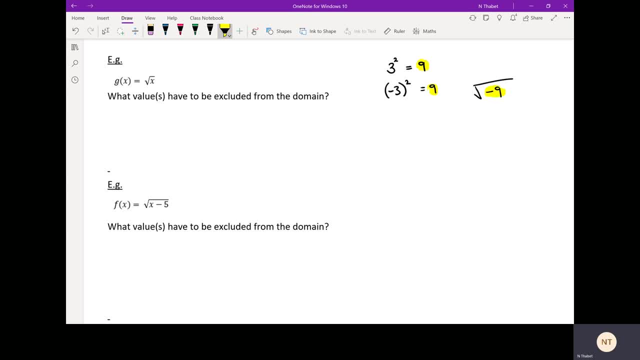 So you cannot have a negative number inside the square root. If you put negative 9 inside the square root And put it into your calculator once again, you will get a maths error. So what are the values more than 1, that have to be excluded from the domain? 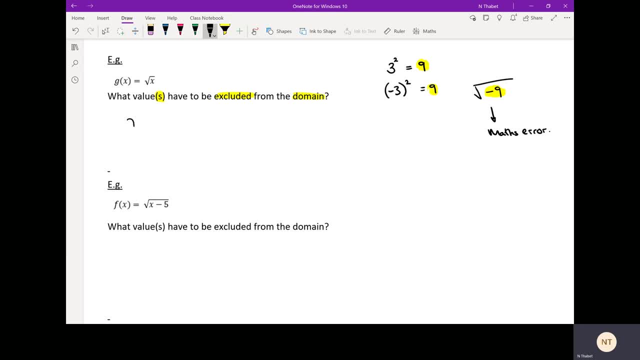 All negative numbers. X cannot be smaller than 0.. All negative numbers Are excluded. You can write- because this is quite a simple question- with just an X inside the square root. you can write: all negative numbers are excluded. But the way to write this is to say X is smaller than 0.. 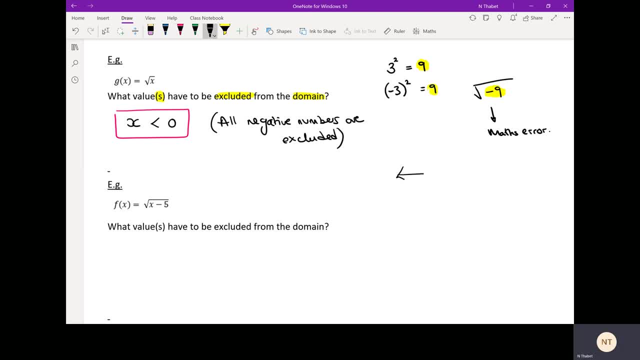 Anything smaller than 0, which means negative numbers. remember, on a number line, this is 0,. this is bigger than 0 and it's getting positive. And this is smaller than 0 and it's getting negative. And this is smaller than 0 and it's getting negative. 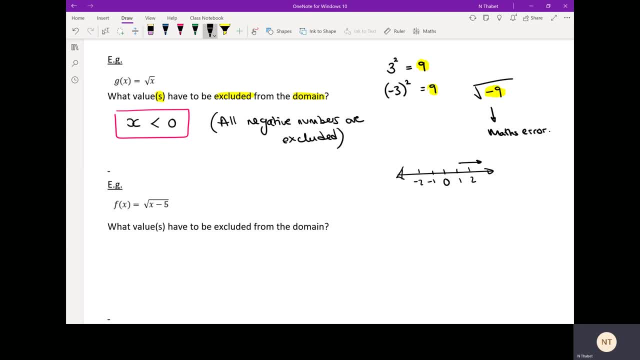 So X is smaller than 0 means all negative numbers are excluded. The fourth example is still a square root and X minus 5, the whole value of what's inside the square root- cannot give us a negative. So we start off instead of an equation that equals to 0, we start off with an inequality. this whole thing. 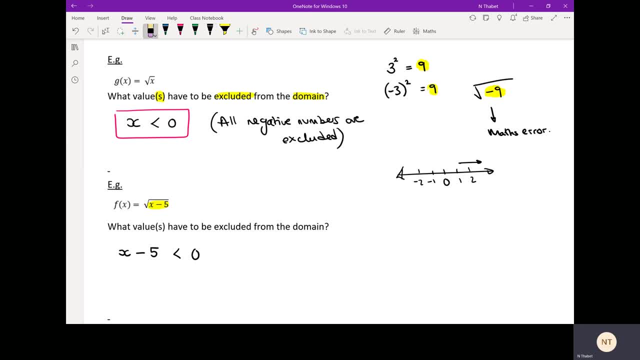 cannot be 0. This cannot be smaller than 0, cannot be negative, And I start by reversing the negative 5, so I add 5.. And now I have the answer: x is smaller than 5.. Anything that's smaller than 5 is going to give us a negative value. Let's check Something smaller than 5,. 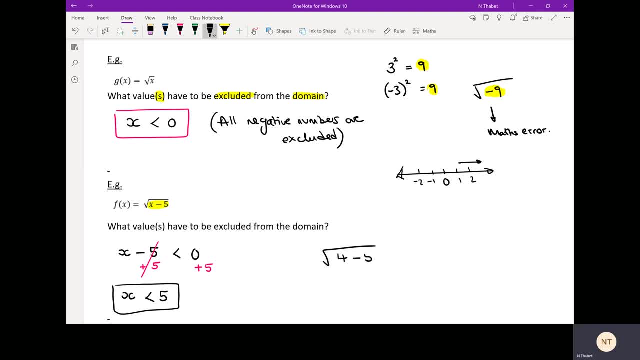 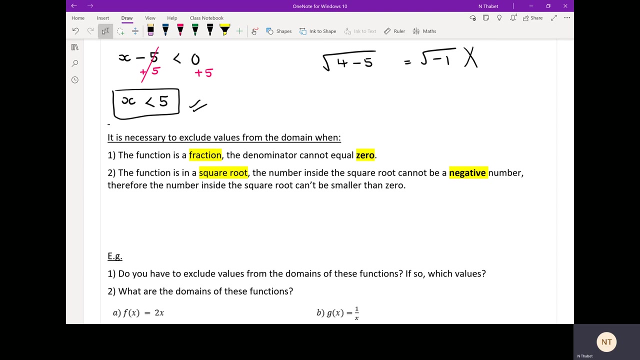 let's try 4.. 4 minus 5 gives us the square root of negative 1, which will not work. So this is correct. Any number smaller than 5 is going to give us a negative inside the square root. So these are the rules. It is necessary to exclude values from the domain when there are. 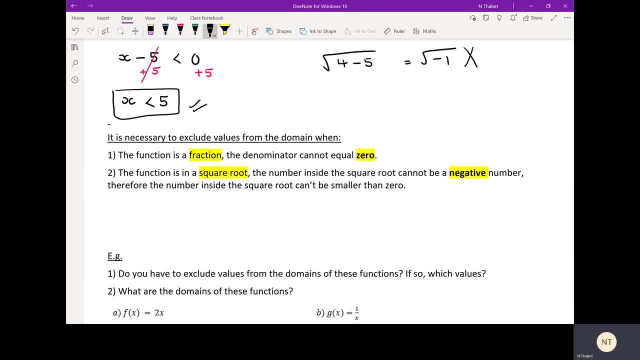 two situations: When the function is a fraction and the denominator- it doesn't matter what the numerator is- but when the denominator cannot equal to 0. The function is in a square root. the number inside the square root cannot be negative. Therefore, the number inside the 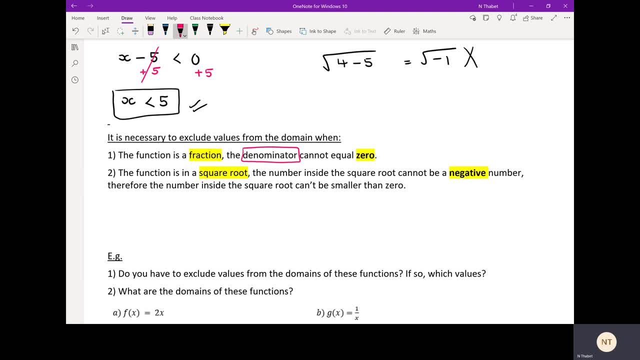 square root can't be smaller than 0. So one of the equations you're going to solve is going to be an equal to 0. The other one is going to be a smaller than 0. And so the result is negative. So that's 1 by 3 plus 1 to give you a зrr. 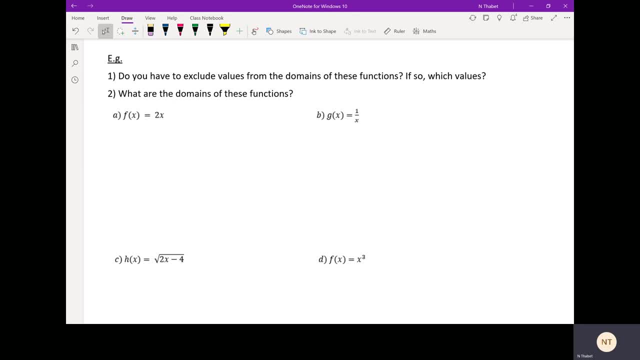 Now let's look at the next few examples. The first question says: do you have to exclude values from the domains of all of these functions- And there are six functions to consider- And if you do, which values do you have to exclude? 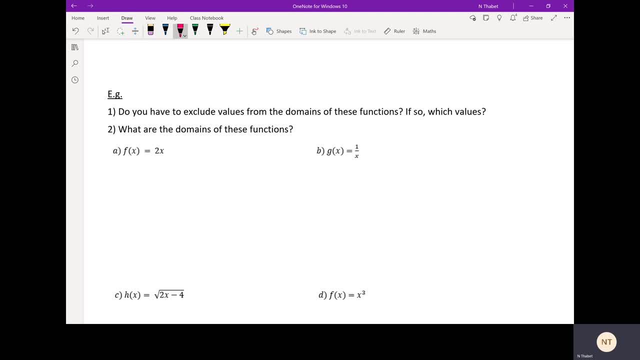 And the question also wants you to tell you, to you to say, to give the domains of these functions. So let's start with the first function, the function of 2x. Will I have to exclude any values? Well, values are excluded when there's a fraction or a square root. 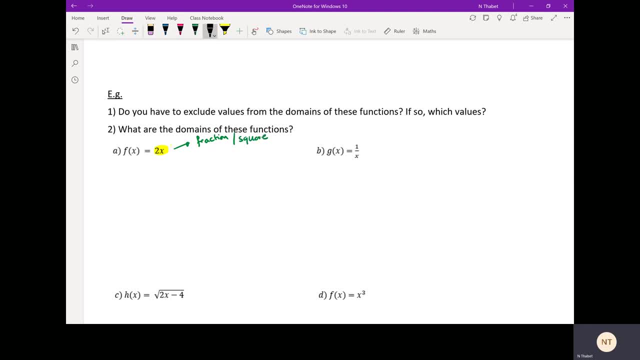 So no values are excluded because they don't fit into these two options. No values are excluded. So that's the answer to question one. If no values are going to be excluded, what are the domains of the function? What's the input? 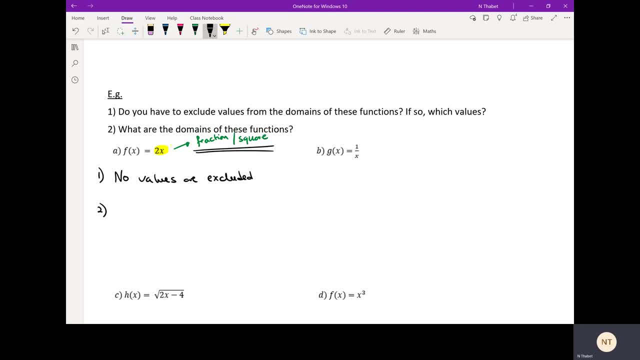 Well, all numbers are possible. So, all real numbers, All real numbers. The domain is all real numbers. Now for part B, it's a fraction, It's exactly as the first example. So, yes, values are excluded. Well, one value is x cannot be zero. 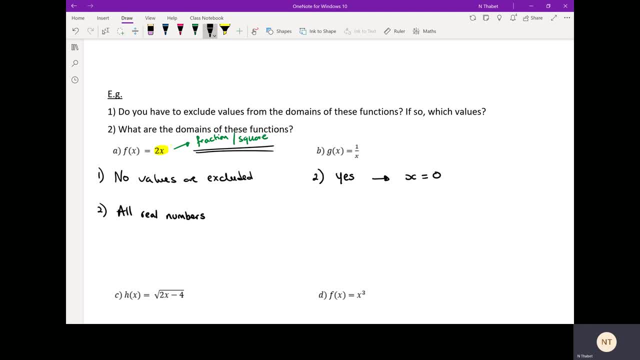 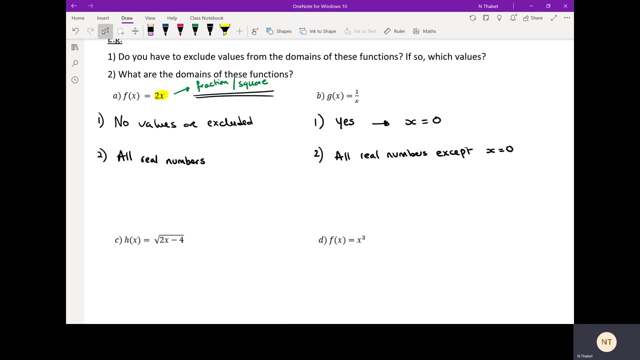 x equals zero is excluded. Let's put that as number one, because we're answering question one And question two: what are the domains? Well, the domain is all real numbers, Except x equals zero. Part C: do we have to exclude values? 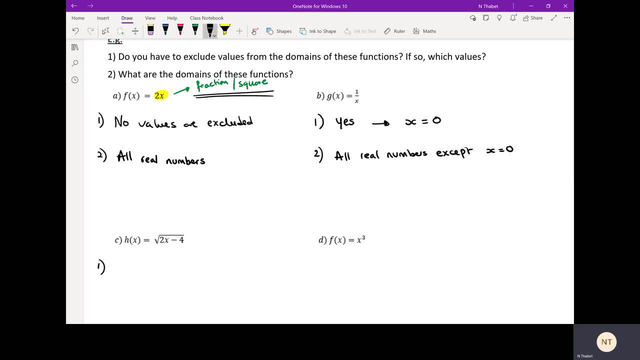 Yes, we will have to exclude values because it fits, It's in the square root. So, yes, some values will be excluded. How do we find which values? Well, we solve as an inequality: 2x minus 4 can't be smaller than zero. 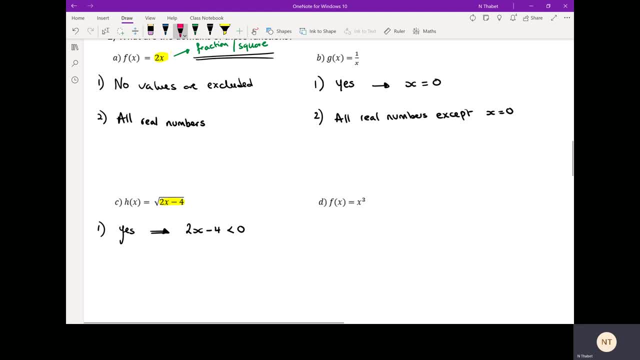 because I can't have negative numbers inside the square root. So I'm going to add 4 to both sides, So that gives me 2x is smaller than 4.. I divide both sides by 2. So that gives me x is smaller than 2.. 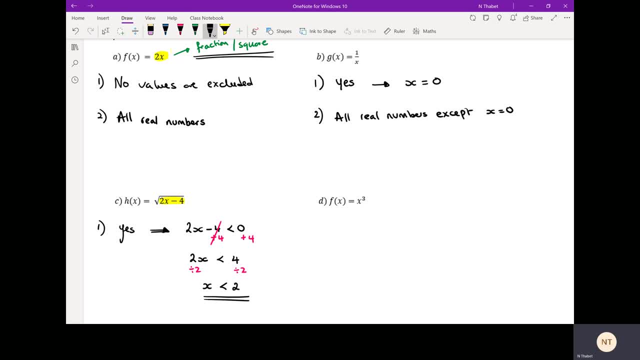 So all numbers smaller than 2 will be excluded. So what is the domain in that case? Well, if that's the excluded, the domain is, of course, what's included. So anything bigger than 2 is included. Now my question is: do you think 2 is included? 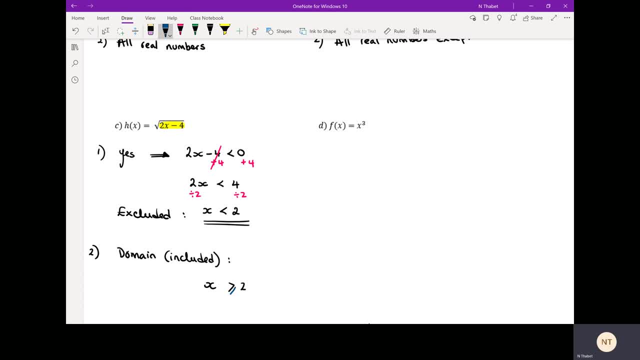 So will I put an equal? Do I put an equal to the inequality or not? Well, let's try. If you're not sure, try The square root of 2 times 2, because, remember, 2x means 2 times x. 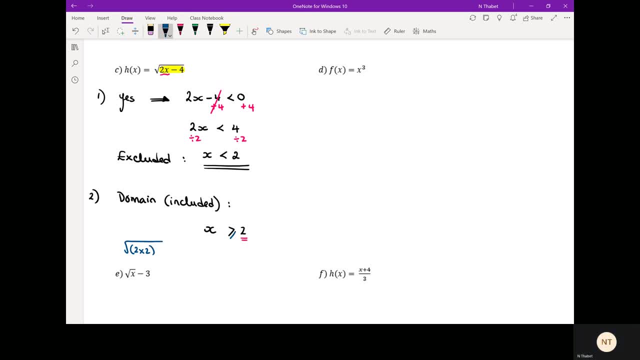 and I'm trying. whether x equals 2 fits 2 times 2 minus 4 gives me the square root of 4 minus 4, which is the square root of 0.. And 0, square root of 0 is 0.. 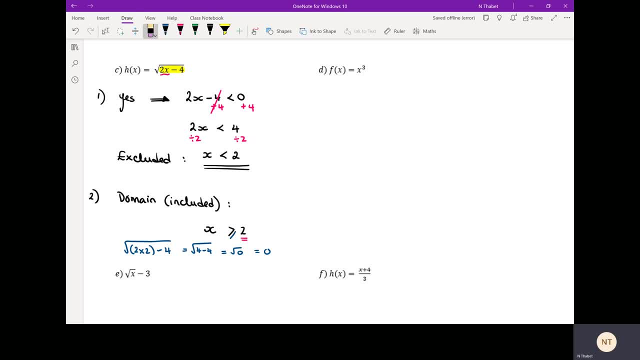 Not a mathematical. That's error. So the number is allowed to be 0. It's not allowed to be smaller than 0. So, yes, 2 fits. So, actually, what are the values in the domain? It's anything bigger than or equal to the number 2.. 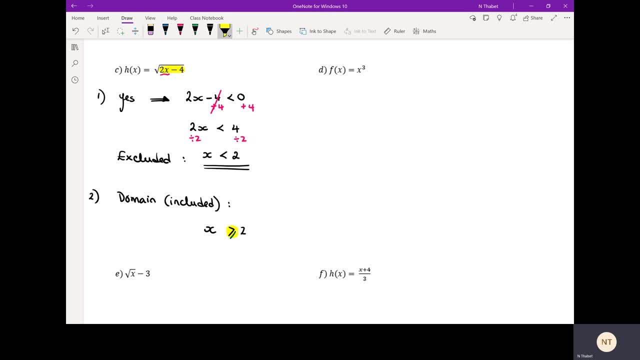 Now for part d this function. do I need to exclude anything from the domain? No, Why? Because it's not a fraction and it's not inside a square root. So what are the numbers included in the domain? All real numbers. 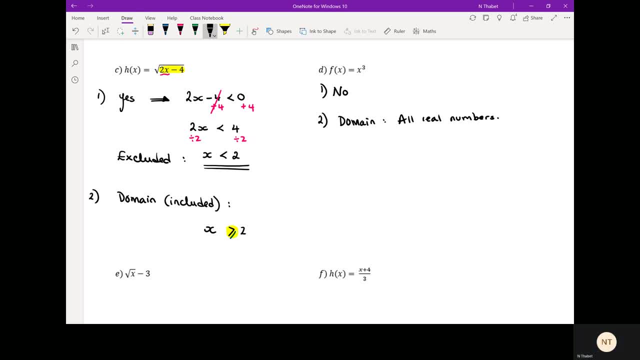 All numbers. Now notice for part e that the square root is only square root. It's not square rooting the minus 3. So you have to deal with that on its own. So yes, there will be values excluded from the domain. 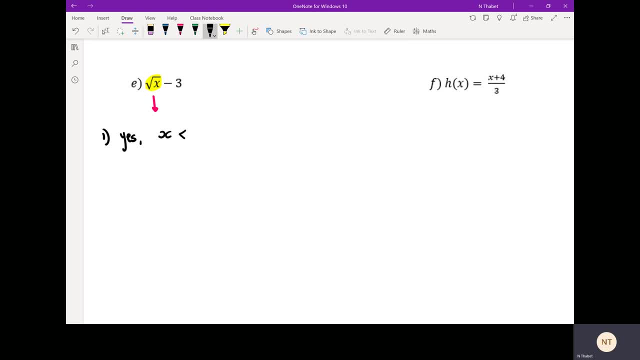 and it's going to be any value which is less than 0,, all negative numbers And 2,. what are the values of the domain? It's anything where x is bigger than or equal to 0. So we can't have any negatives, anything smaller than 0,. 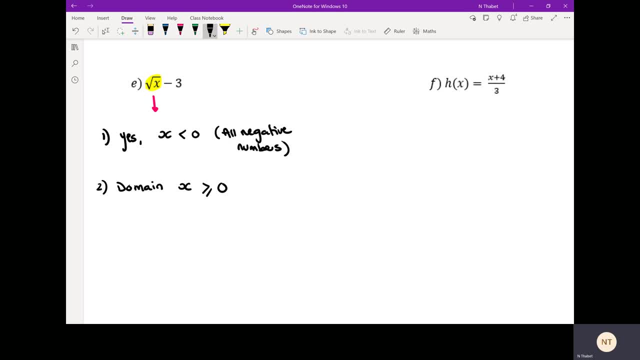 but we can have. x is bigger than or equal to 0.. And then the last example, example f. do we have to exclude anything from the domain, The domain of this function? Well, it looks like it's a fraction, but the denominator doesn't have an x. 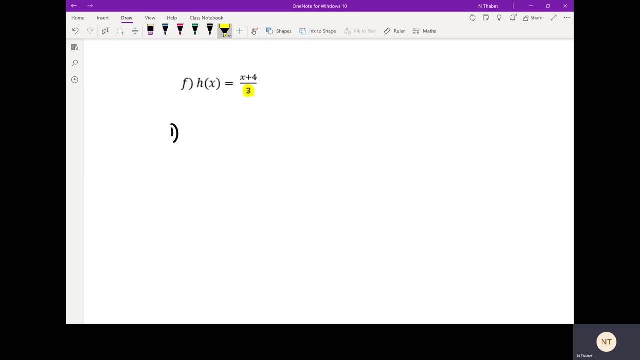 So I'm never going to divide by 0. It doesn't matter about the numerator. The numerator can be 0. That's fine, And the denominator doesn't have an x, so it's always the same. I'm always dividing by 3.. 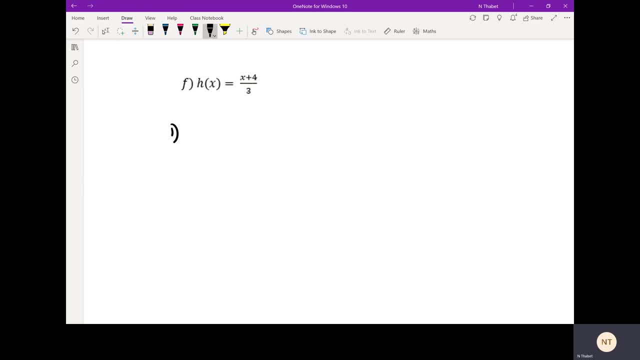 So actually, that's not the kind of fraction that we're interested in. So, no, no values. Values have to be excluded. So what is the domain of this function? What's the input? The input is all real numbers. Now, what I would like you to do is to pause the video. 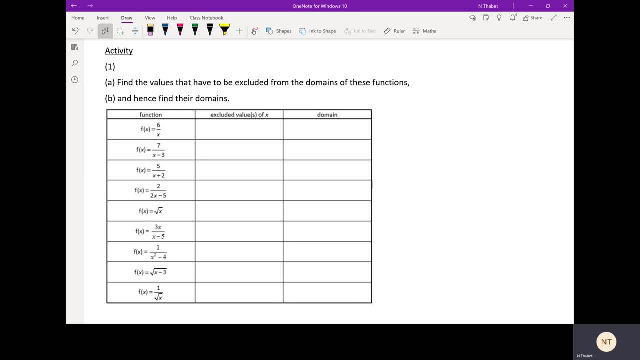 and to try these questions on your own. I am then going to go through the answers, But it's important that you take the time and have a think about these before I go through them, because I'm not going to do the same with those. 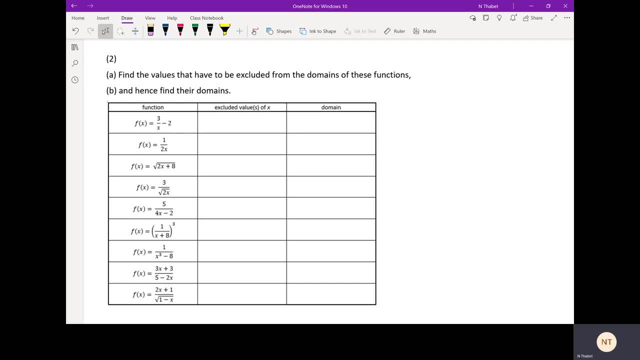 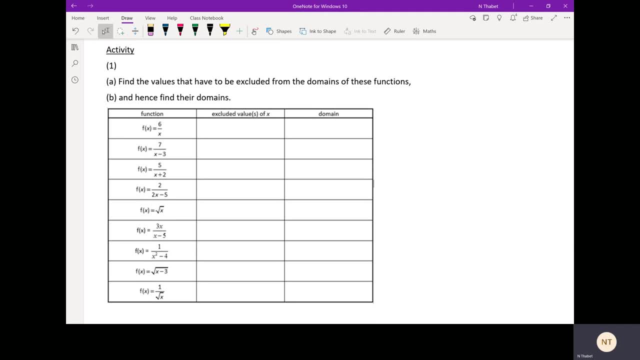 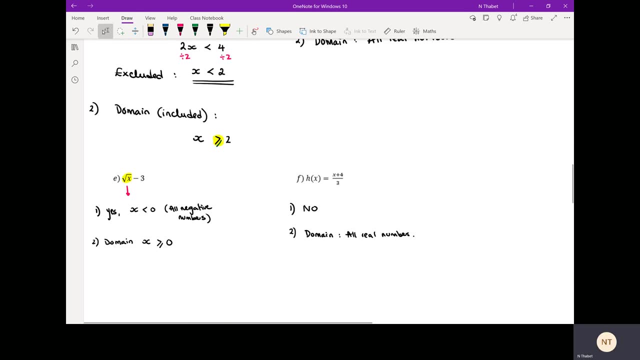 These are the questions that you're going to do completely on your own, and we will mark them in class. So pause the video because I'm going to start going through. These are exactly like the examples that I've just talked you through, Except all of them. 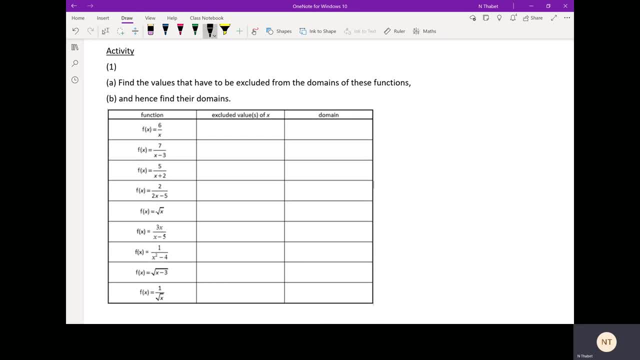 there will be values excluded. So you have to find the values excluded and then you have to find the domain. This is a fraction. X cannot be zero, So the values excluded is x equals zero And the domain is all numbers except x equals zero. 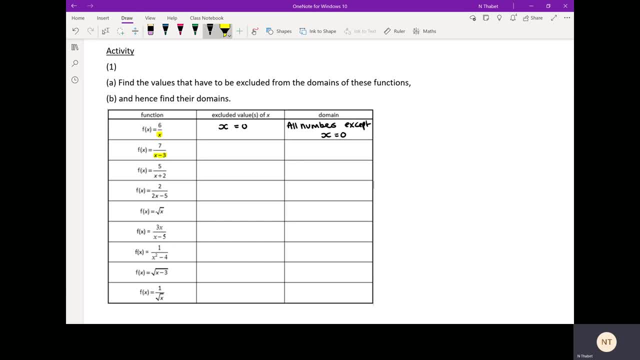 The second function is also a fraction, And x minus three can't equal to zero. Therefore x equals a positive three, because of course I add three here and I add three there. That's the value that is excluded. So all numbers are part of the domain, except x equals three. 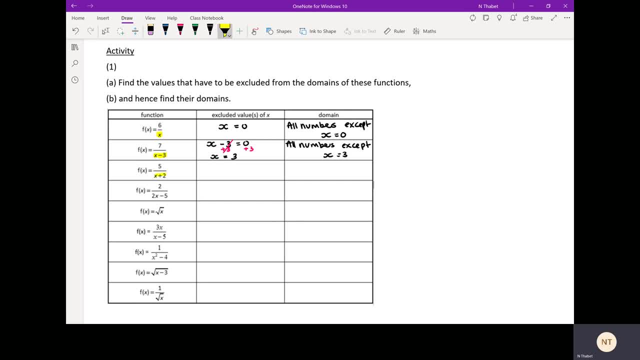 Again, this is a fraction. So x plus two cannot equal to zero. So the number that's excluded is x equals minus two, And again it's. all numbers are part of the domain, Except x equals minus two. This is also a fraction. 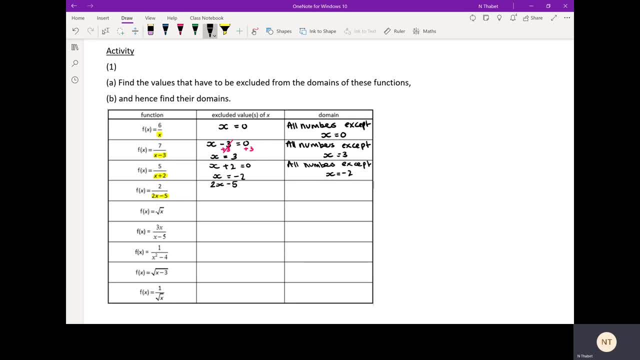 And again it's. all numbers are part of the domain, except x equals minus two. So two x minus five can't equal to zero. I'm going to add five to both sides and divide by two, So x cannot be five over two. 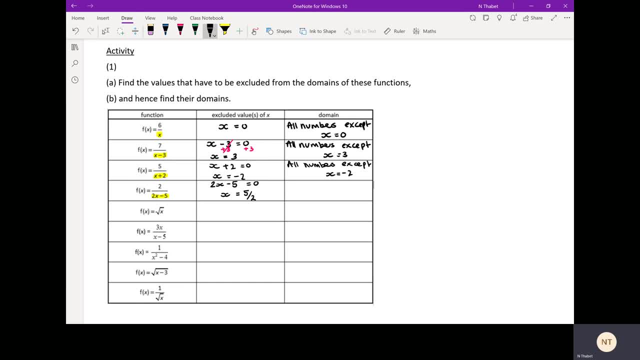 You can also write it as a decimal. That's the value that's going to be excluded. So the domain- the numbers that are included are all numbers except x- equals five over two. We get to this question and we start dealing with square roots. 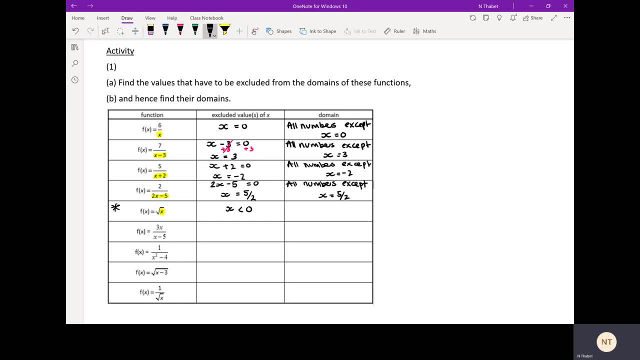 So x cannot be a negative number. x cannot be smaller than zero. So the domain is all the numbers which are bigger than or equal to zero. We are allowed to have a zero inside the square root. Then we have another fraction, We have a negative number. 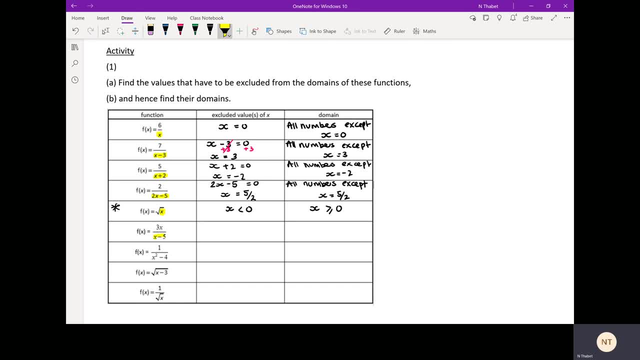 We have a square root, We have another fraction And it is the denominator that we care about. We don't really care about the numerator. So it is the x minus five that cannot equal to zero. So x equals a positive five is the value that has to be excluded. 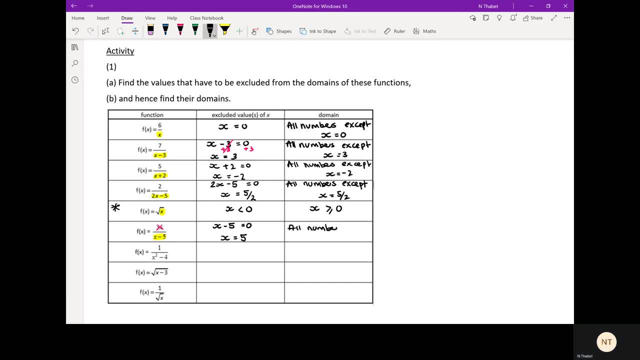 So the domain is all numbers except x equals five. So the domain is all numbers except x equals five. x equals five. We have another fraction, So I've got x squared minus four can't be zero, So I'm going to add four to both sides. 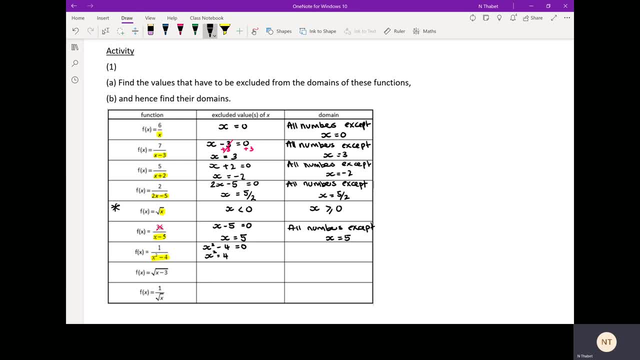 So I have x squared is a positive four And x. remember, when you square root- because I'm going to square root to get x- you actually get the x, two values, a positive and a negative, because 2 squared gives us 4, but also negative 2 squared. 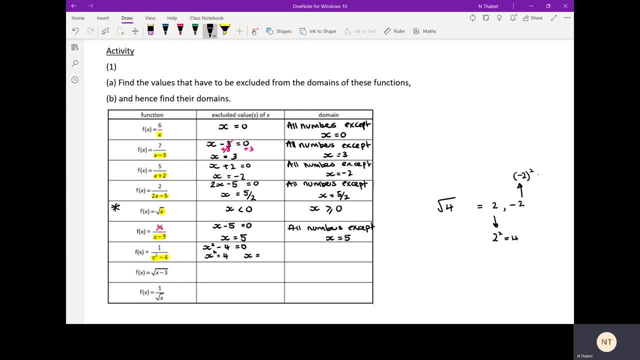 gives us a positive 4.. So there are two values that x cannot be, because if x takes the value of 2 or negative 2, and you square it, you get a positive 4, you take away 4, you get a 0.. 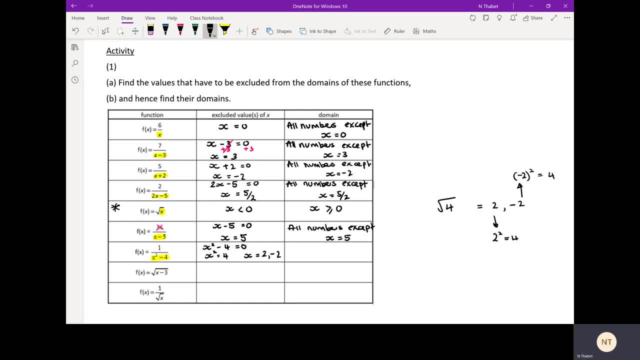 So it's 2 and negative 2.. So what are the values that are part of the domain? all numbers, all real numbers, except x is 2 and x is negative 2?? Both of these cannot be part of the domain. 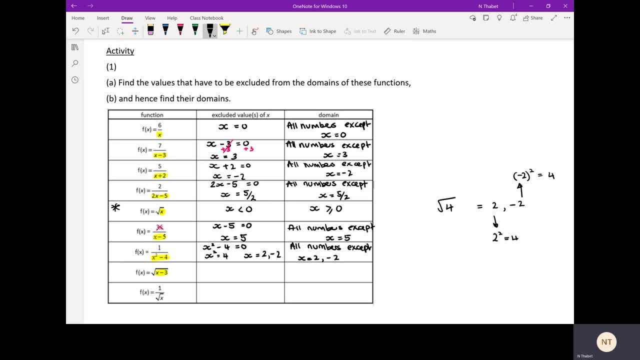 And then I've got inside. the square root is x minus 3.. So x minus 3 cannot be smaller than 0, cannot make a negative number. So x is smaller than 3 is excluded. Anything smaller than 3 will give a negative number. So what's the domain? The domain is all numbers where x. 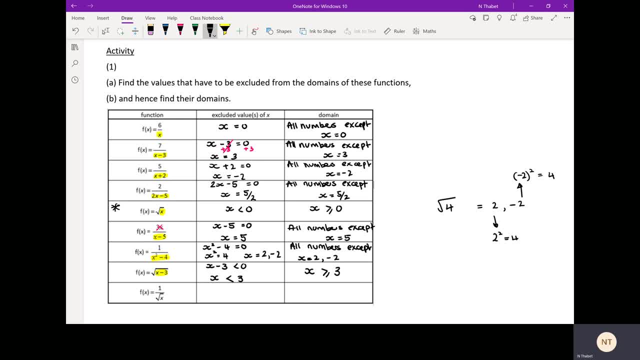 is bigger than or equal to 3,, because 3, if it's equal to 3, will give us 0.. 3 minus 3, 0. And we're allowed to have a 0 inside the square root. Now, finally, the final question. 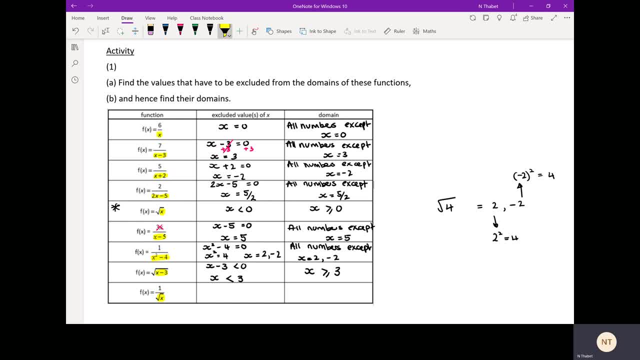 has both a fraction and the square root. So x cannot be 0, that's for sure, because I cannot divide by 0 and the square root. So even though 0 is normally allowed inside the square root, the square root of 0,.